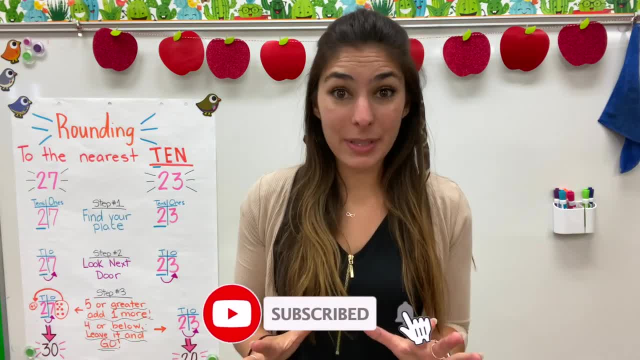 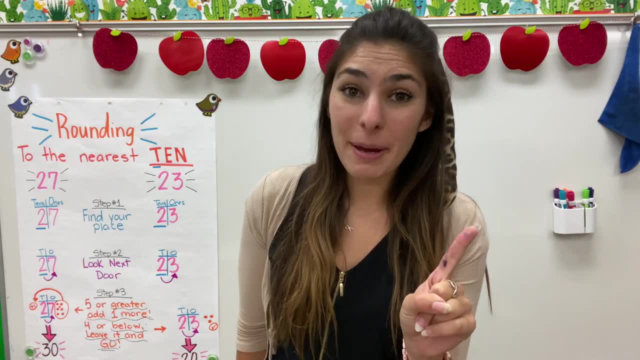 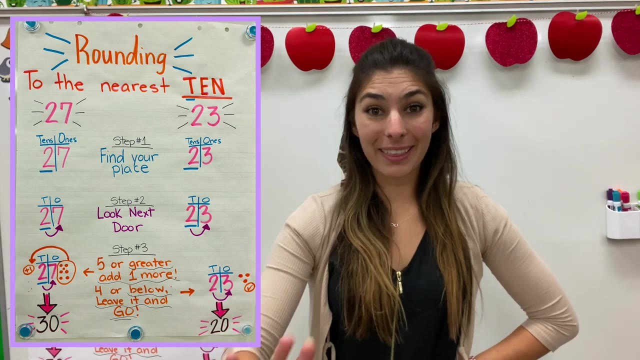 Hey friends, welcome back to Bloomin' with Ms B. Today we are talking rounding, So there are a couple ways that we can round to the nearest 10.. First is by following a fun little rhyme: Find your place, look next door. five or greater. add one more Four below: 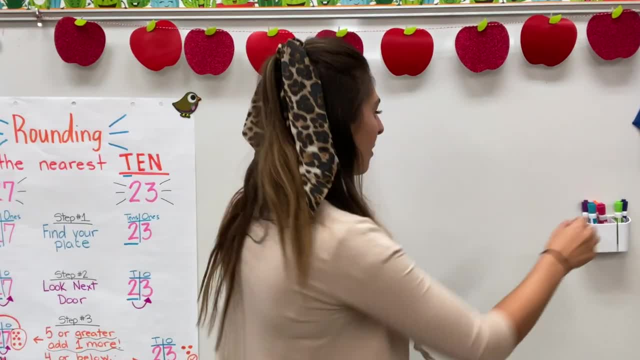 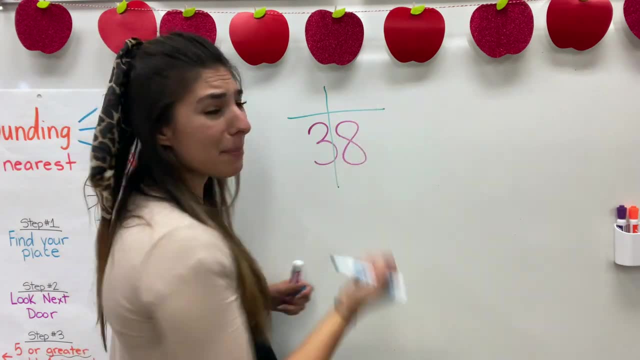 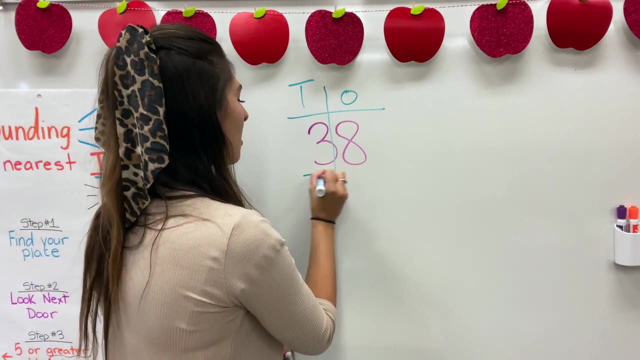 let it go. So let me show you one while following that rhyme. So if we have the number 38. Step one is going to be find my place, and that means place value. So we always start with our ones and because we're rounding to the nearest 10, we're going to underline the number in the tens. 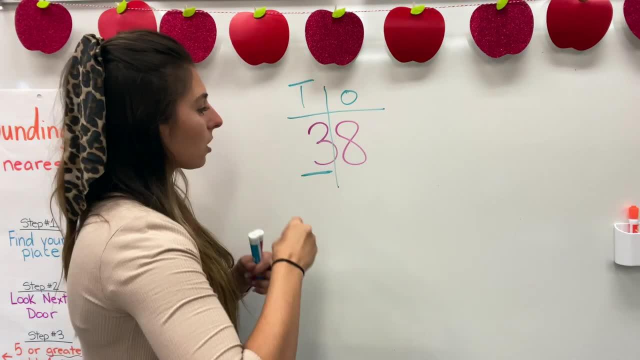 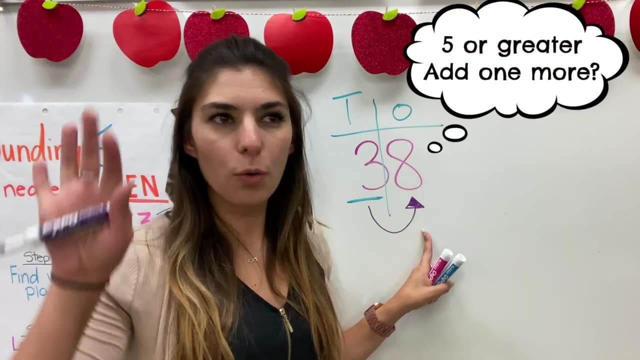 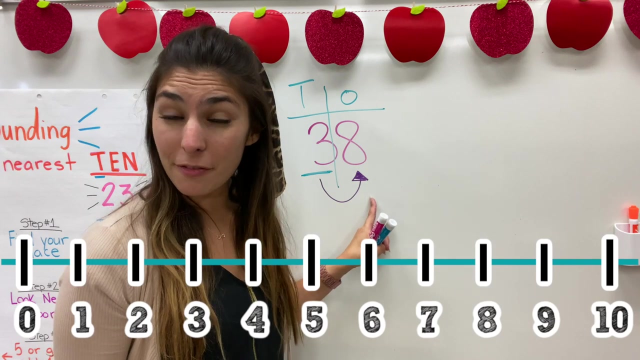 place, which is the three. Now I'm going to look next door, which is going to be at the eight. So I'm going to look at this eight and ask myself: is this five or greater? add one more or four below. let it go So. is eight greater than five or less than five? 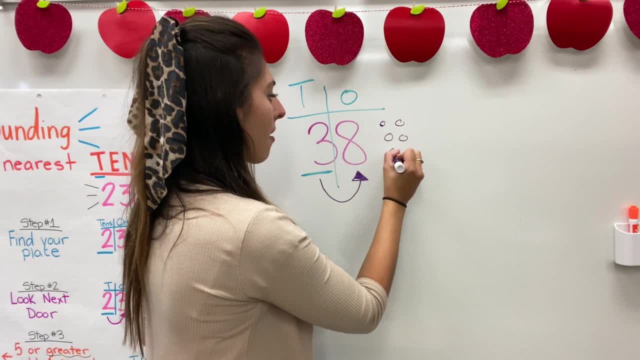 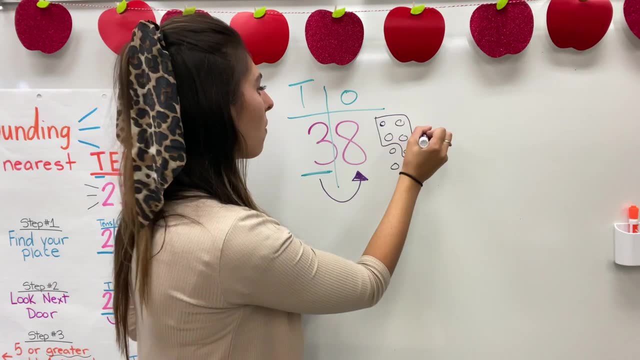 Well, let's see if I have one, two, three, four, five, six, seven, eight. One, two, three, four, five, There's five. It's much more than five. So I'm going to add one more. So what is? three plus. 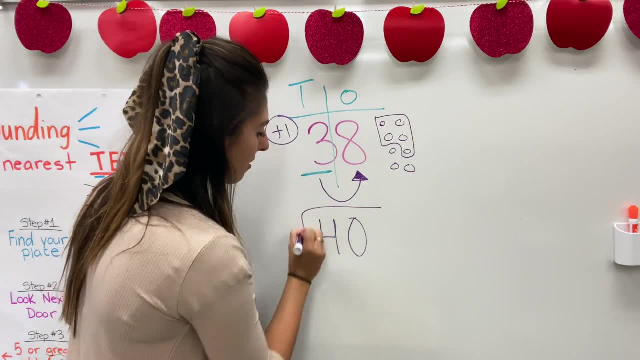 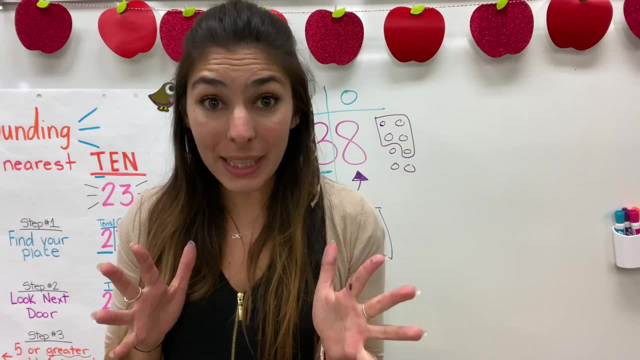 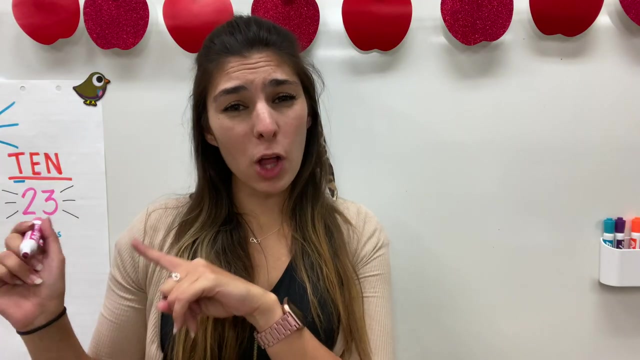 one Four, and then that's going to turn to zero. We round 38 to 40. Also because it's closer to 40 than it is to 30. We can really see this by making a number line. I'm going to do a totally different number, still following that rhyme, but this time doing more of a 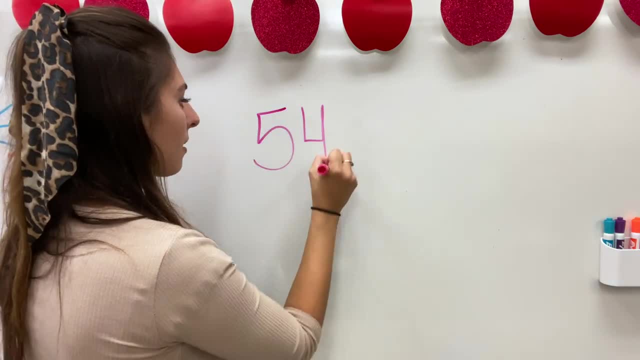 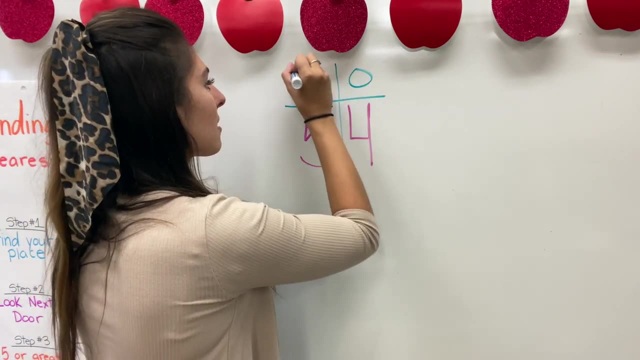 number line. So this time let's make it 54.. Step one: I need to find my place, So I'm going to draw my two chart: Ones tens. We are rounding to the nearest 10. So I'm going to underline: 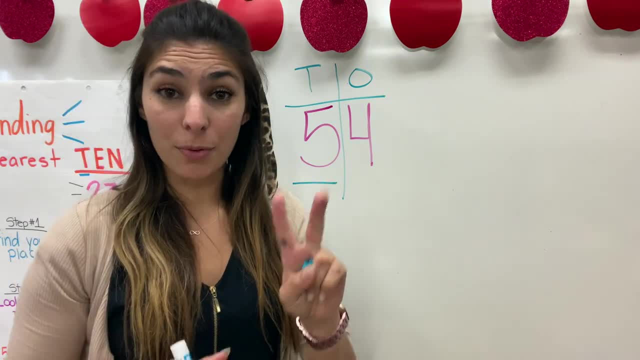 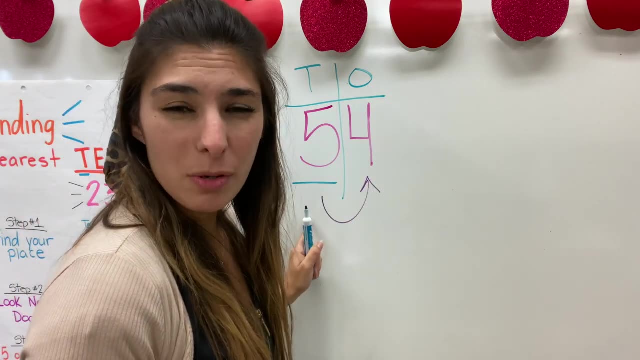 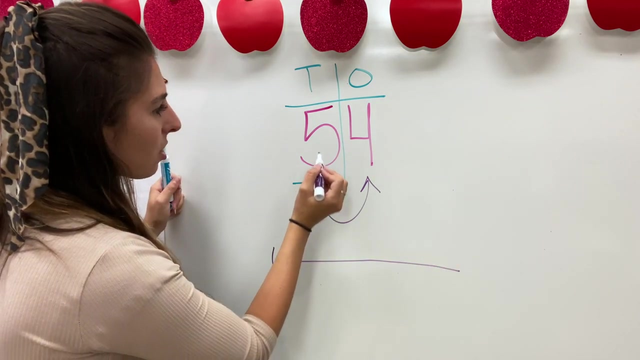 the number in the tens place, which is the five. Now step two: look next door. So I'm going to look next door at this four. but I'm also going to look next door as far as making a number line. So I'm going to draw my number line here and whatever number this is, So this is five, but this is five. 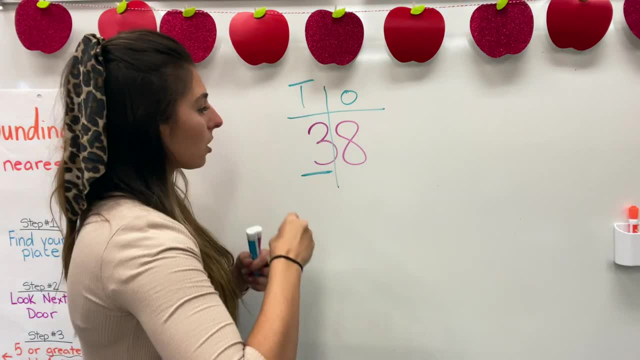 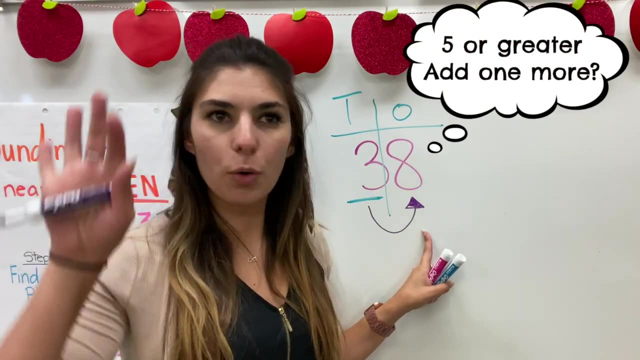 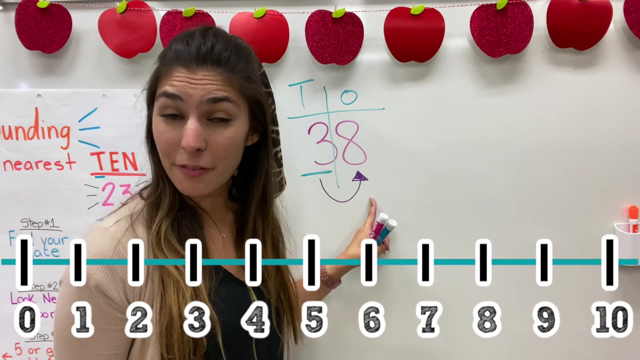 place, which is the three. Now I'm going to look next door, which is going to be at the eight. So I'm going to look at this eight and ask myself: is this five or greater? Add one more or four below. let it go So. is eight greater than five or less than five? 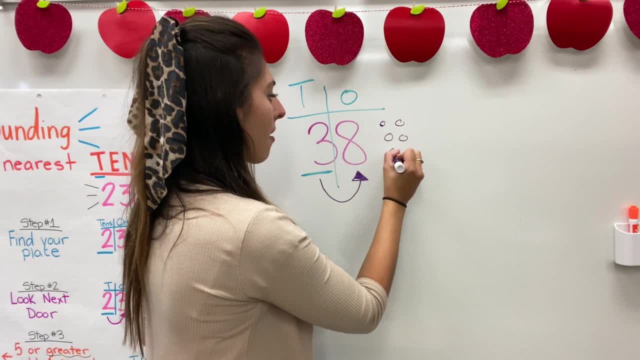 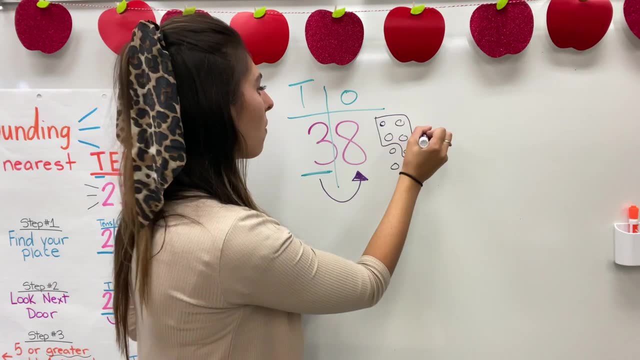 Well, let's see if I have one, two, three, four, five, six, seven, eight. One, two, three, four, five, There's five. It's much more than five. So I'm going to add one more. So what is? three plus. 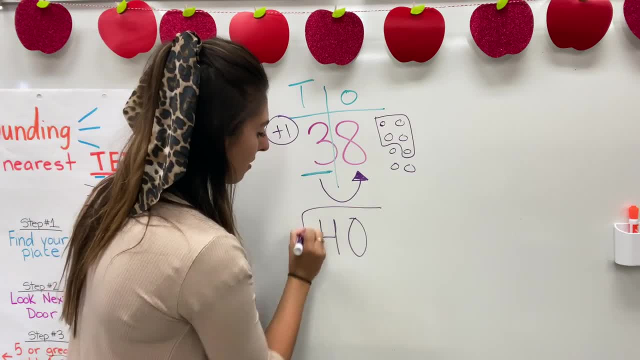 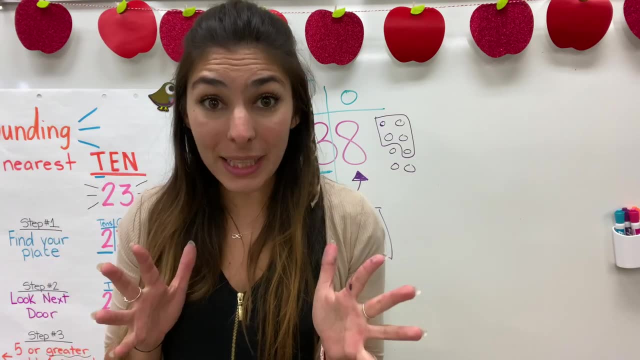 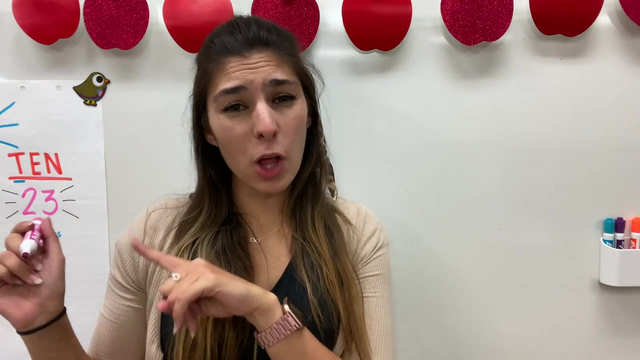 one Four and then that's going to turn to zero. We round 38 to 40. Also because it's closer to 40 than it is to 30. We can really see this by making a number line. I'm going to do a totally different number, still following that rhyme, but this time doing more of 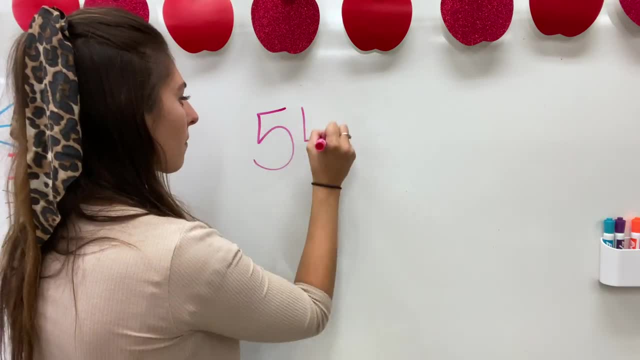 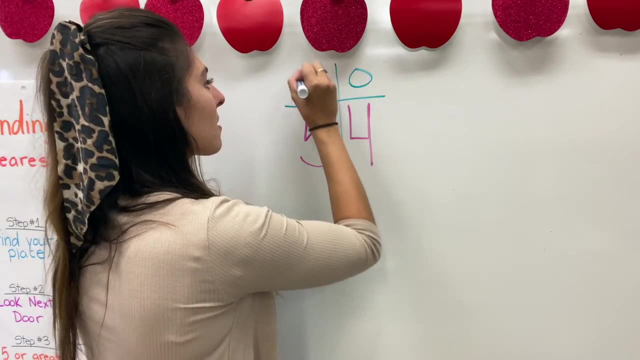 a number line, So this time let's make it 54.. Step one: I need to find my place, So I'm going to draw my two chart ones, tens. We're rounding to the nearest 10. So I'm going to underline: 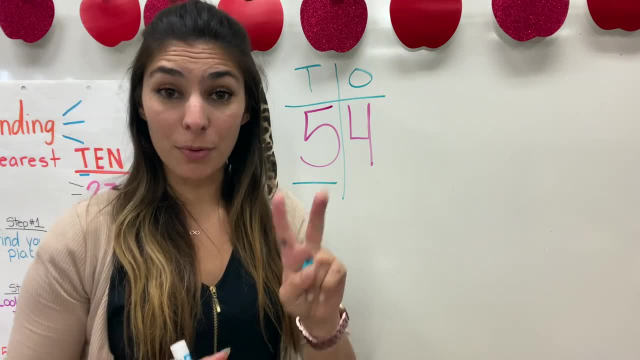 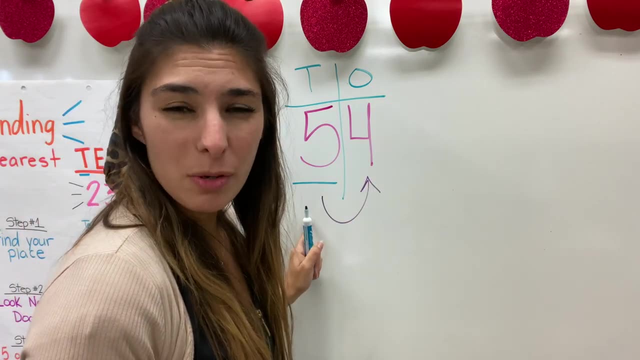 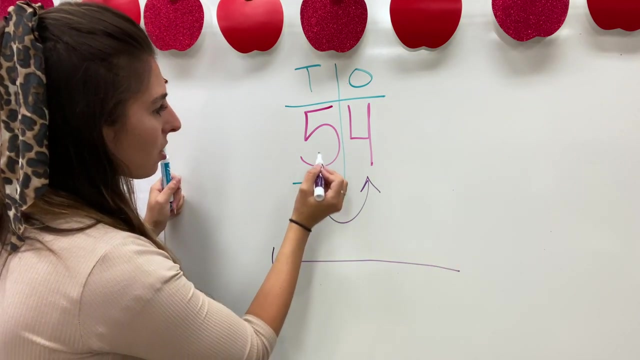 the number in the tens place, which is the five. Now step two: look next door. So I'm going to look next door at this four. but I'm also going to look next door as far as making a number line. So I'm going to draw my number line here and whatever number this is, So this is five. 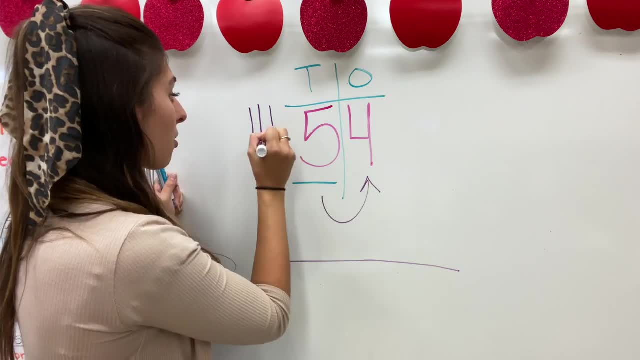 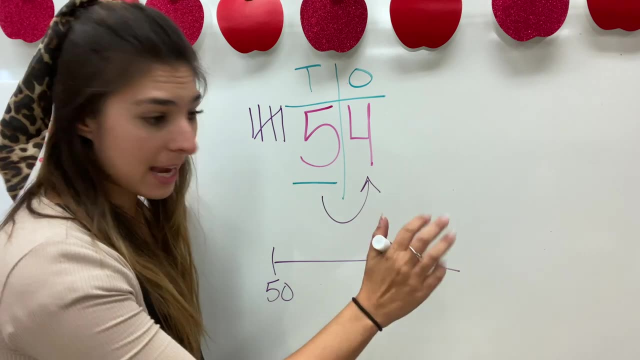 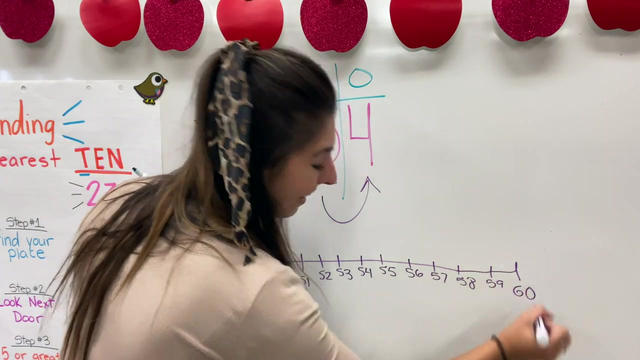 but this is five tens, So technically that's 10,, 20,, 30,, 40,, 50. So we are going to start that number line at 50 and we can only go up 10. So we're going to do So from here. I'm going to see. 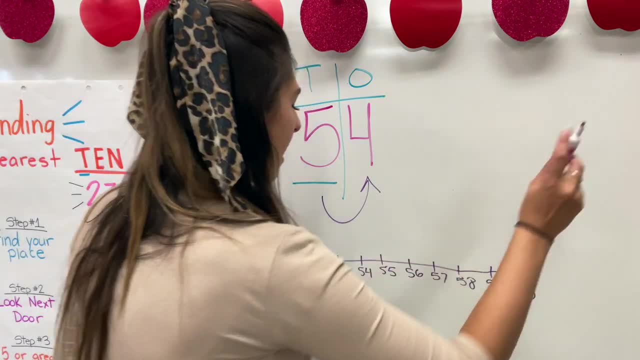 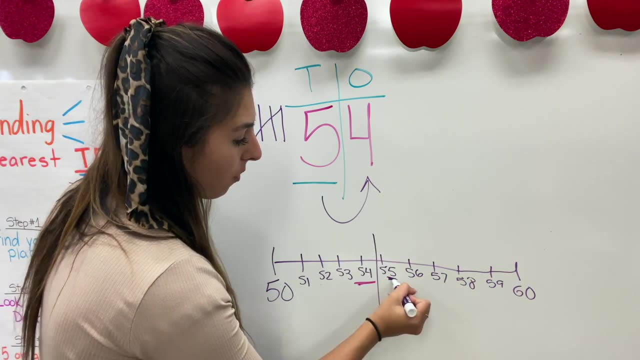 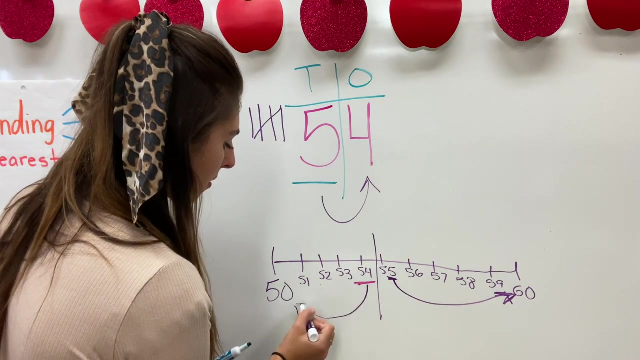 54. That's my one. So I see here here is 54 and actually anything over that, five or more, five or greater. add one more four below. We're going to let it go. We can also just see that this four is closer to 50 than it. 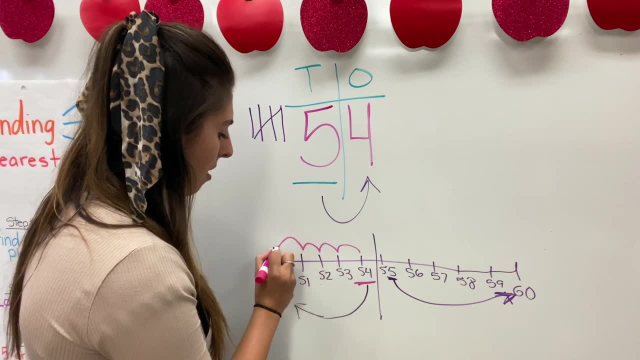 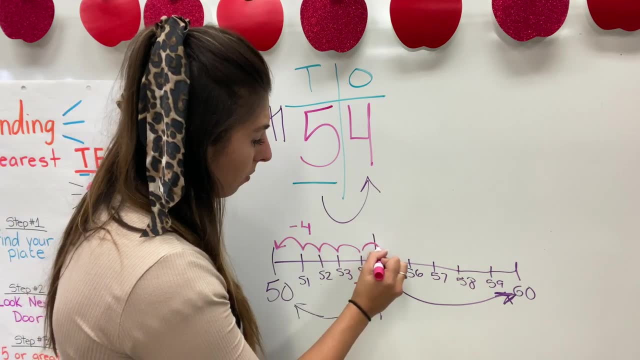 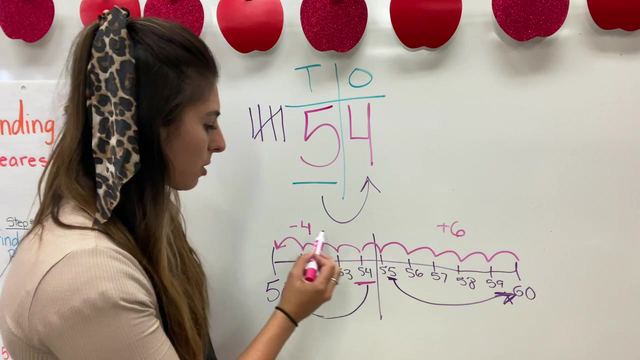 is to 60. So if we go one, two, three, four, so that only takes four hops backwards. Well, if we went forward, it would take one, two, three, four, five, It would take six, and we want to go the shortest way possible, So we're going to.